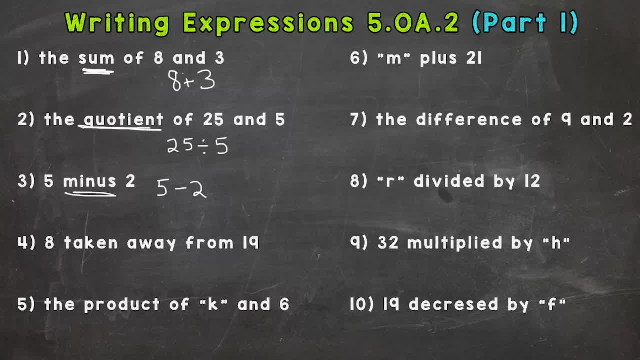 I should have mentioned this at the beginning, but oh well, I'll mention it now. You can either write these out with me or you can just listen to me as I go through these. Eventually you will get to the mastery check, which is the third video, where you will try some on your own and you can write them. so you can. 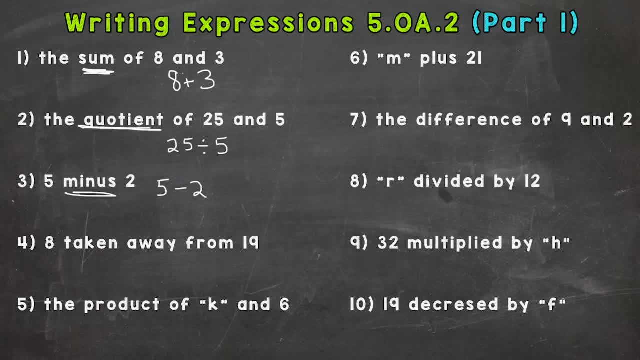 just listen now or write up to you. So number four: 8 taken away from 19.. This is the most commonly missed type of expression here, because we are taking 8 away from 19. so think about it: if you had $19 and you take 8 away, it's actually 19 minus 8, it is not 8 minus. 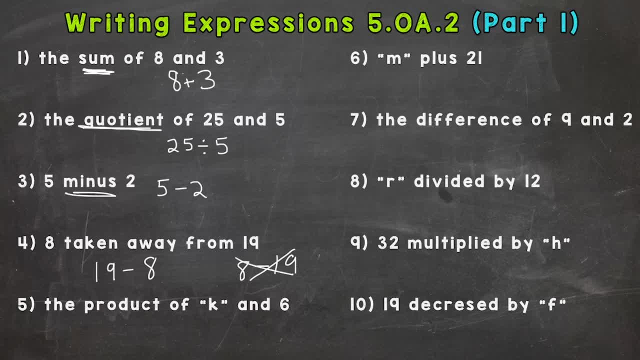 19. order matters when it comes to subtraction and division. so 19 minus 8 right here would equal 11. 8 minus 19 right there equals negative 11. did that give you the same thing? no, obviously not. so you need to think about what is being. 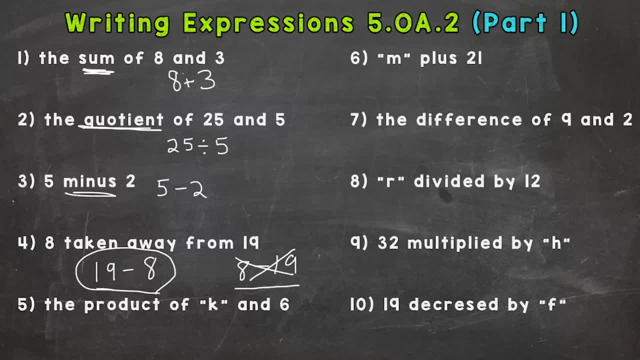 asked. that's one you definitely need to double check and read back to yourself to see if you have it. so that's 19 minus 8. order matters: division, subtraction, now addition and multiplication. those are commutative, which means the order doesn't matter. so take a look back up at number one. we 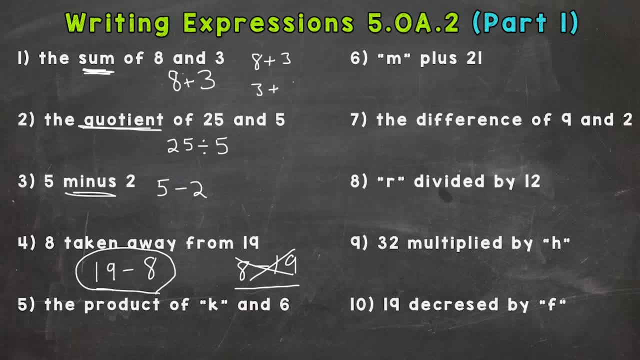 have 8 plus 3. let's switch the order and see if we get the same thing. so 8 plus 3 is 11, 3 plus 8: 11. that will work for any addition problem. you switch the numbers, you get the same answer. same for multiplication: 3 times 2 is 6. 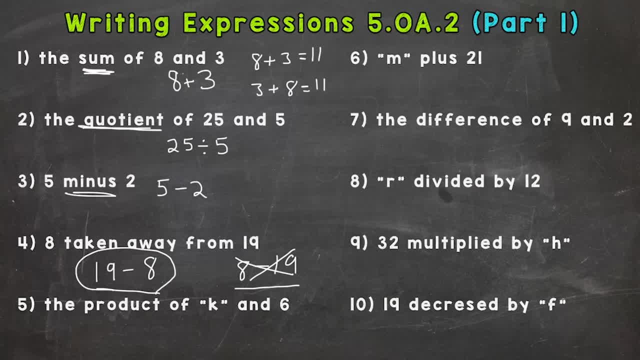 8 plus 3 is 11. that will work for any addition problem. you switch the numbers, you get the same answer. same for multiplication: 3 times 2 is 6, 2 times 3 is 6. so let's go down to number 5, the product of K and 6. no, that is. 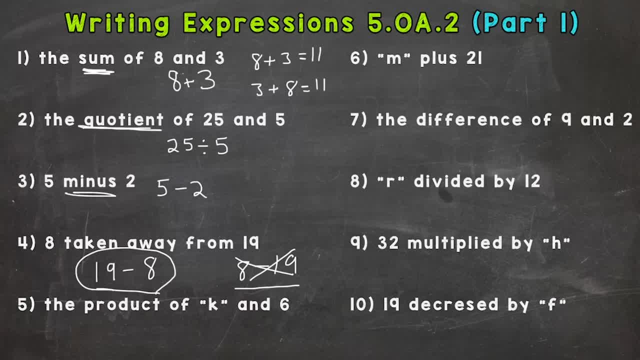 not a mistake. we are supposed to have a letter in our math problem there. so we have a K and a 6. so I'm gonna explain a little bit about what a letter means in the math problem. this is actually a little bit of algebra here. a letter in a. 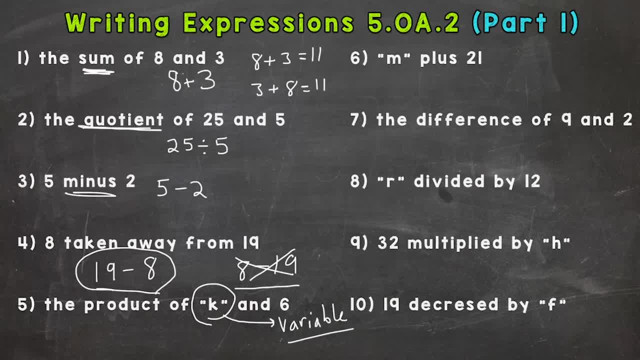 math problem is called a variable. It means a missing piece, like the missing puzzle piece to the math problem, And it can be any number in the world. That K can be a hundred, it could be two, it could be a million. We don't know what it is. So when we write out, 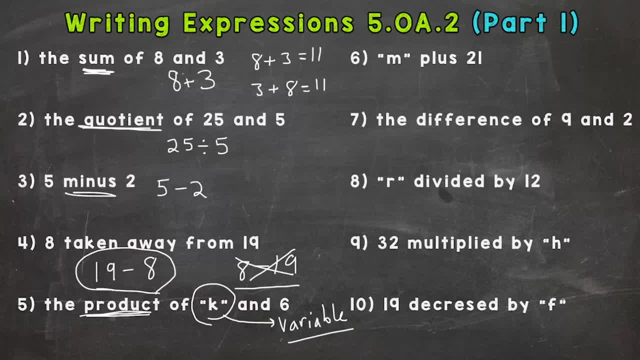 product of K and six. product means multiplication K times six. So that right there in the bottom left-hand corner would be okay because we're just starting out. But we don't want to use an X for a multiplication sign when we are working with algebra problems because we don't know if that's a multiplication or 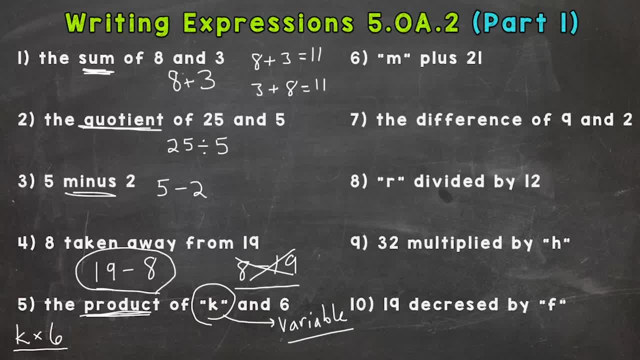 an X, That could mean K X six or K times six, So we want to avoid that. The most common thing in algebra is the number run forest Number run forest culinaryucks right next to the letter And usually you will see the number come first. 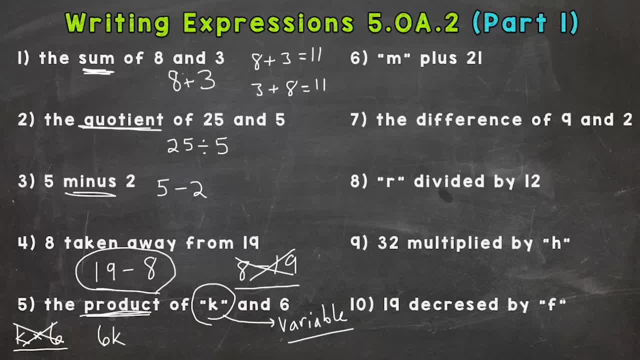 Remember, multiplication is commutative, so you can switch the numbers and letters and still get the same answers. So 6k, that would mean six times k. Another one you can use, or you might see, is right next to a parenthesis. 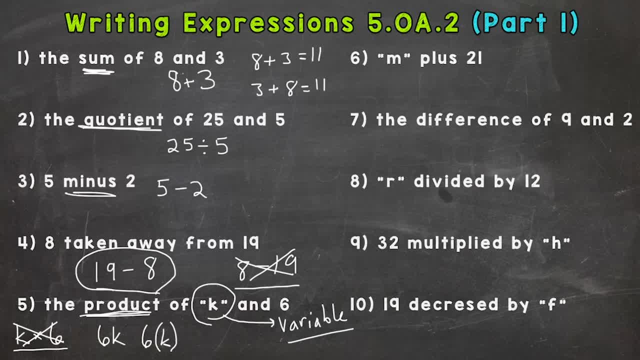 Anything right next to a parenthesis means multiply, so that means six times k. I'm going to come up here, so I have room. Another one is a dot- Make sure it does not look like a decimal, but that means multiplication. And the fourth one is an asterisk: means multiplication. 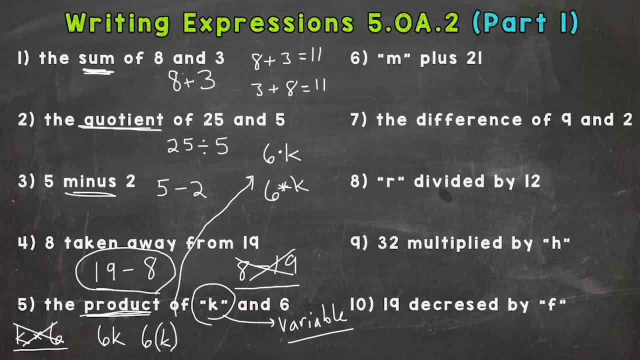 So four new ways to show multiplication, because, remember, if we use an x, we don't know if it means multiply or it's an x. Number six: m Plus 21.. So all we have there is m plus 21.. 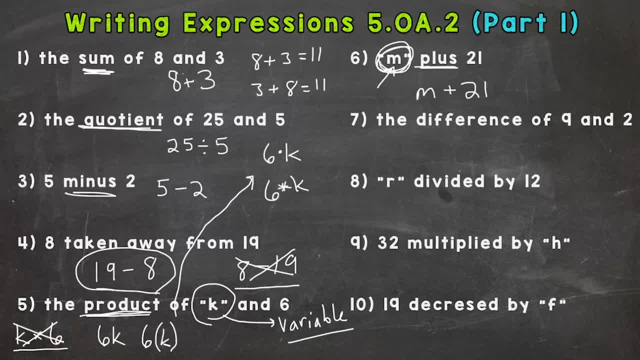 Do we remember what a letter in a math problem is called? If we need to look at the bottom, go ahead and look. Hopefully you said variable- Yes, a variable, And what does it mean? Hopefully you are thinking a missing piece to a math problem.